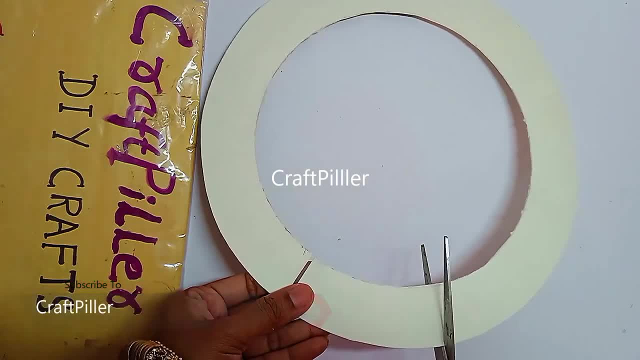 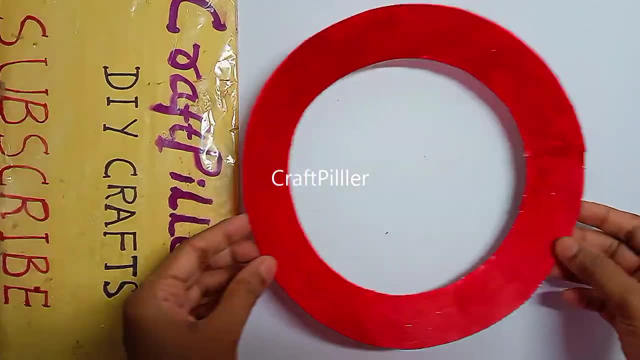 I want to be the greatest Everybody on the fake shit. I look around and feel like everybody is the fakest. I make this every day and I'm impatient, Hoping. one day I blow up from the basement Statement. the top is so vacant Out on your shit that I think is amazing. 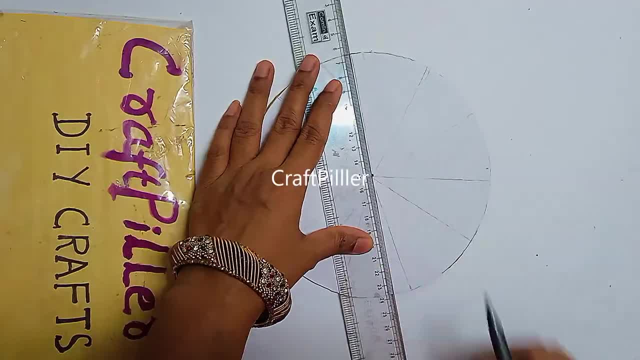 Waiting for my day when I'm playing Sold out shows for a thousand faces. Hey, give me that crown Getting my way and to be put down. It ain't your place, dog. This my town. If I want that shit, then I'll get it right now. 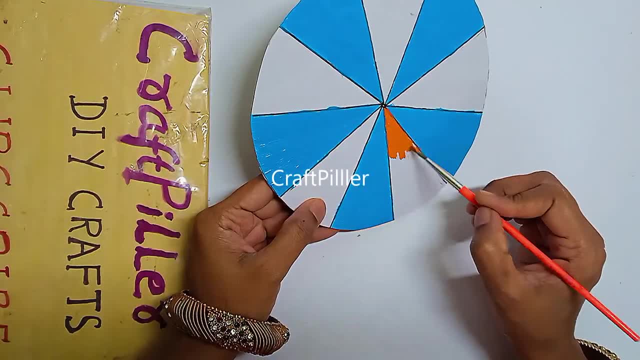 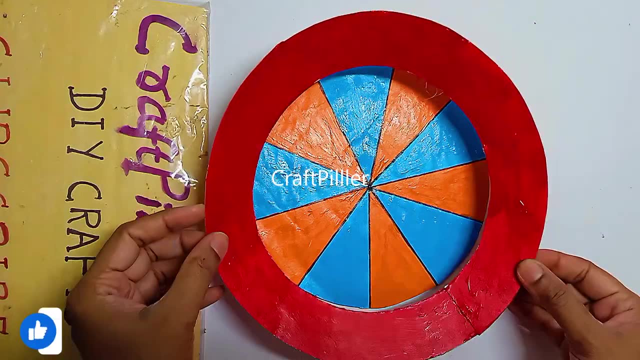 I'm losing it. The noose that fits. I'm losing shit. A stupid myth. If you choose to live or choose to dip, you choose to fight or lose your grip and lose a gift. I feel like I'm losing my mind. Is everybody in the world blind? 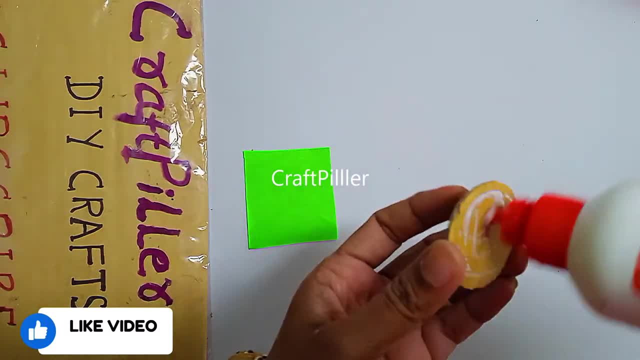 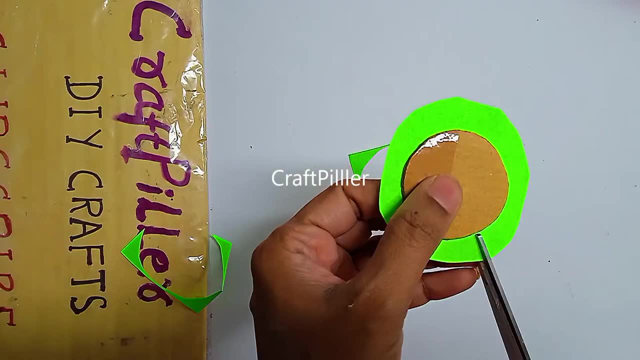 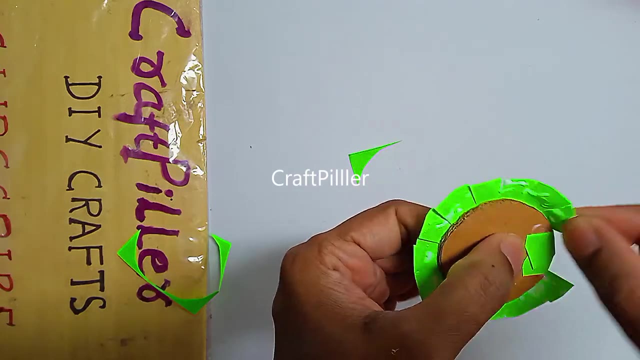 Please, Lord, give me a sign, a sign. I feel like I'm losing my mind. Is everybody in the world blind? Please, Lord, give me a sign, a sign There's no mercy in this world, just hunger, thirsty persons. 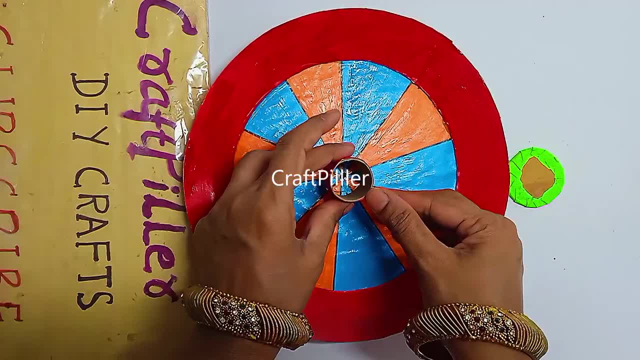 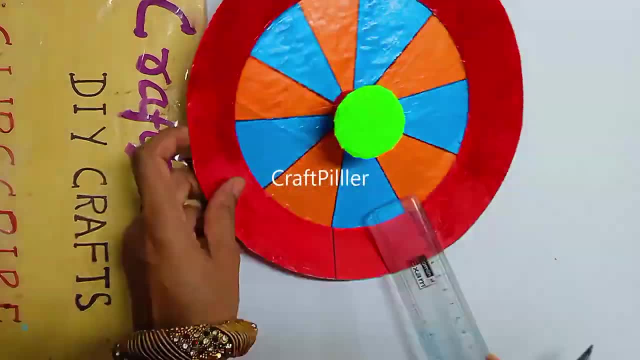 In different versions. each new update, that shit worsens. Why? Pull back the curtain and you'll see the different vermin. We all have different burdens that all seem to cause disturbance. So do me a favor, Don't treat me like a neighbor. 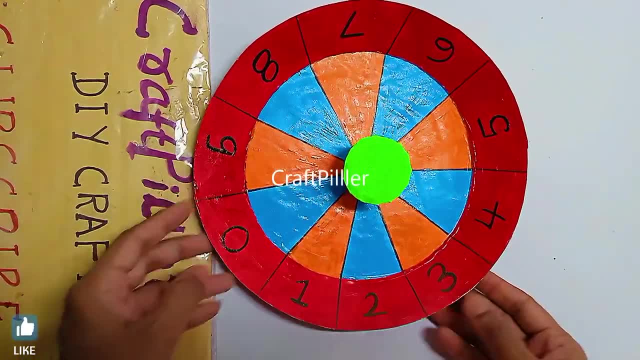 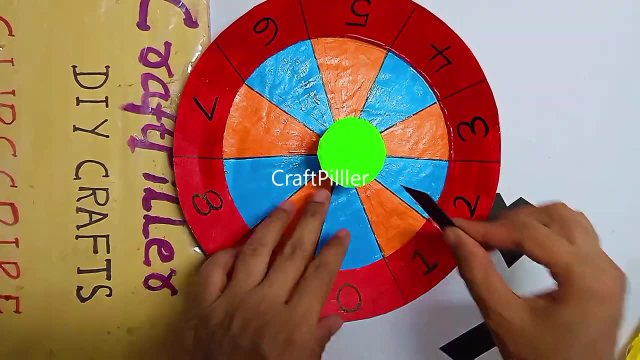 Don't need the different flavors of your problems just to savor. I've got my own issues. I need a comb to get through. Don't need to groan with you, Just go get your own tissue. I feel like I'm losing my mind. 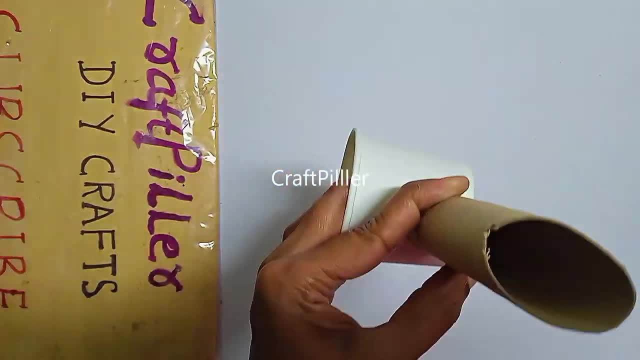 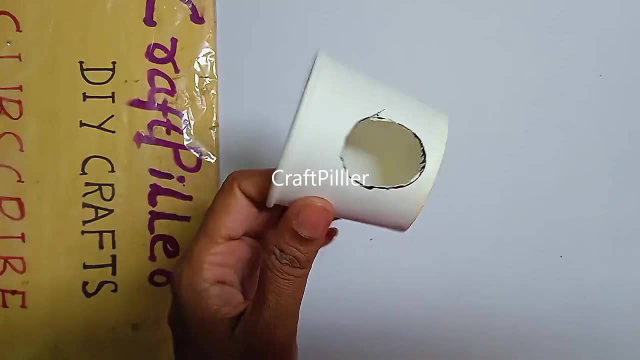 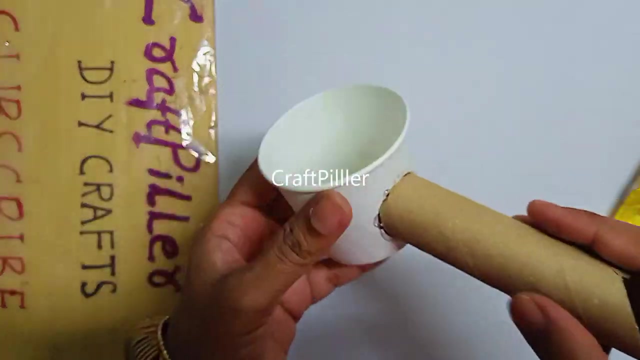 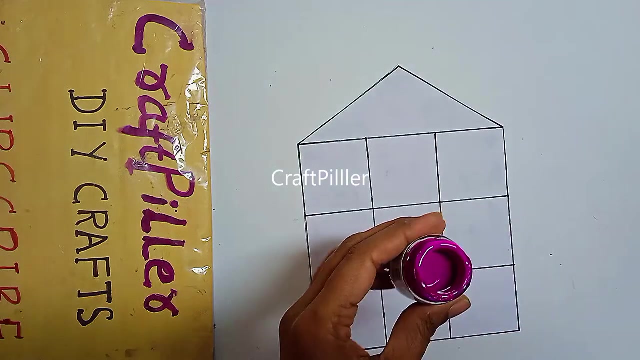 Is everybody in the world blind? Please, Lord, give me a sign, a sign. I feel like I'm losing my mind. Is everybody in the world blind? Please, Lord, give me a sign, a sign That's it the end of the song. Next time you'll sing along. 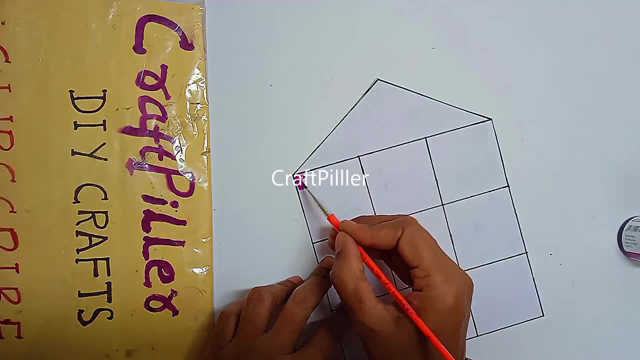 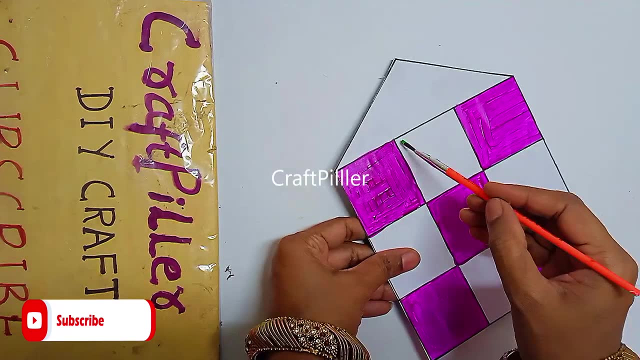 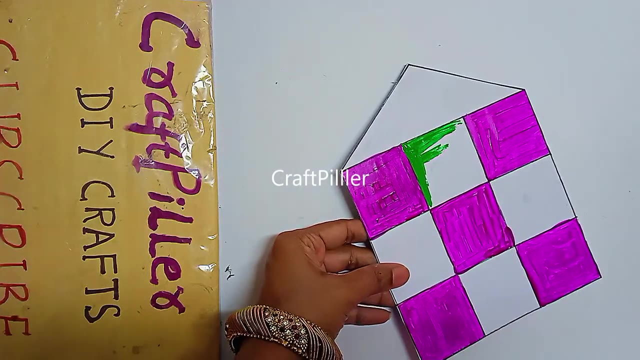 Trust me, there's nothing wrong. I just need to carry on, Cause society's a myth. Put the blame on me there to make you sit, listen to what they give. don't ask questions, shut your lid. yeah, don't ask questions, shut your lid. i need to run away from this and go get off the grid. feel like my brain. 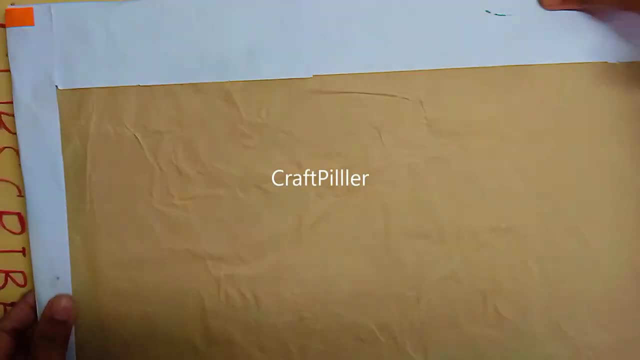 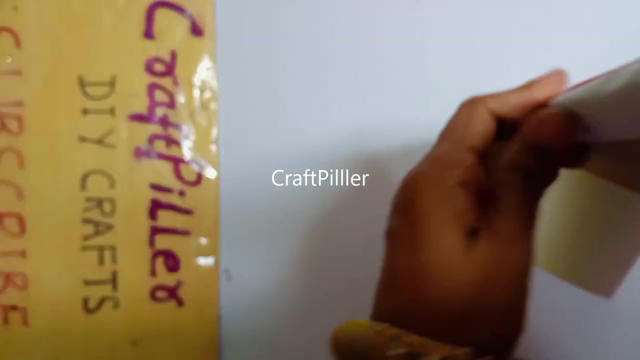 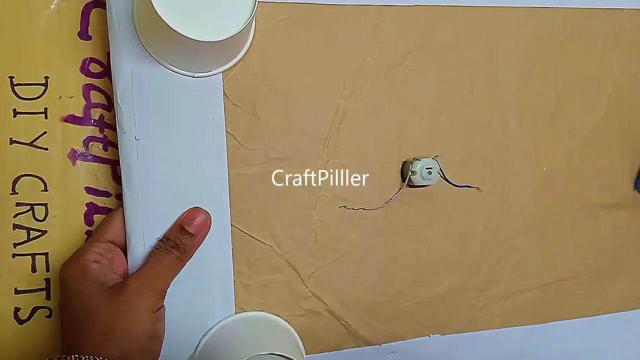 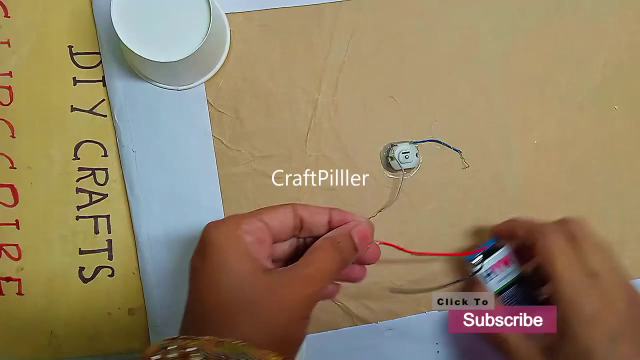 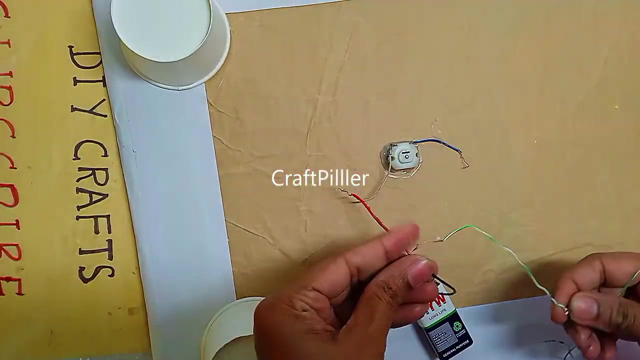 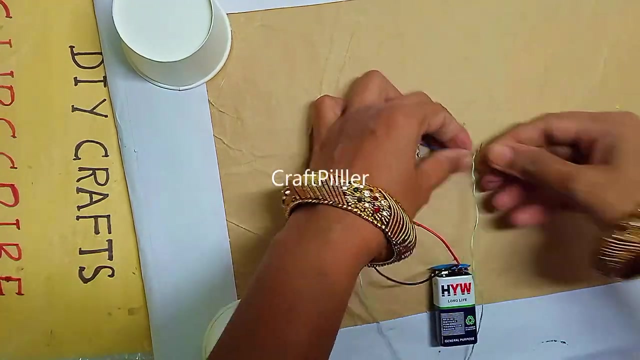 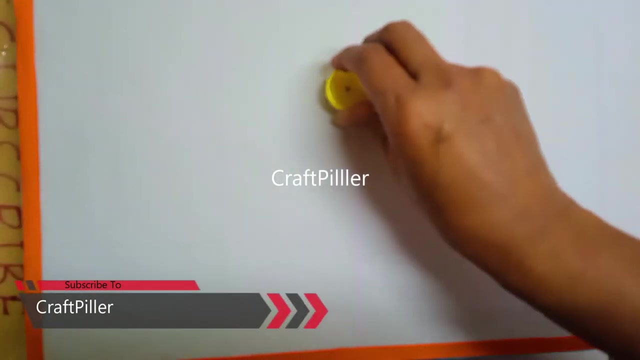 is overloaded, man, i'm losing it. don't let them tell you what to do, man. they don't know shit. i feel like i'm losing my mind. is everybody in the world blind? please, lord, give me a sign, a sign. i feel like i'm losing my mind. is everybody in the world blind? please, lord, give me a sign. 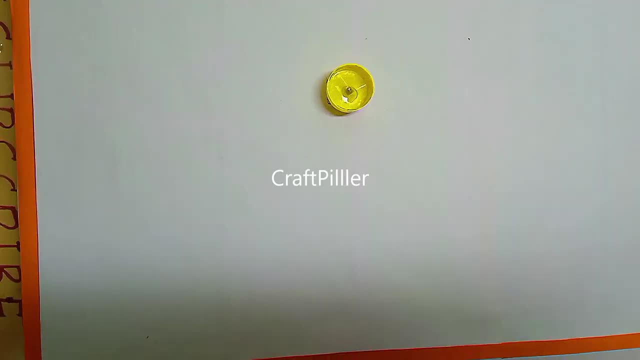 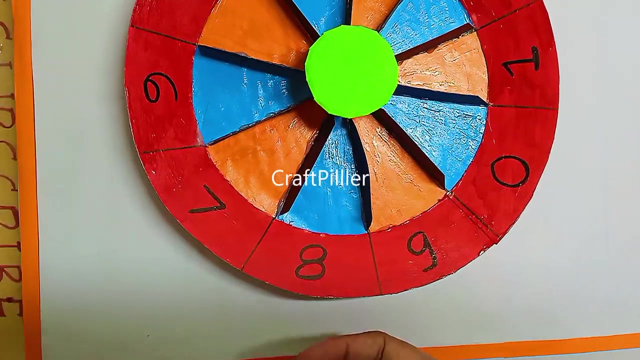 a sign. i want to be the greatest everybody on the fake shit. i look around i feel like everybody is the fakest. i make this every day and i'm impatient hoping one day i blow up from the basement statement. the top is so vacant i don't hear shit. that, i think, is amazing. waiting for my day when 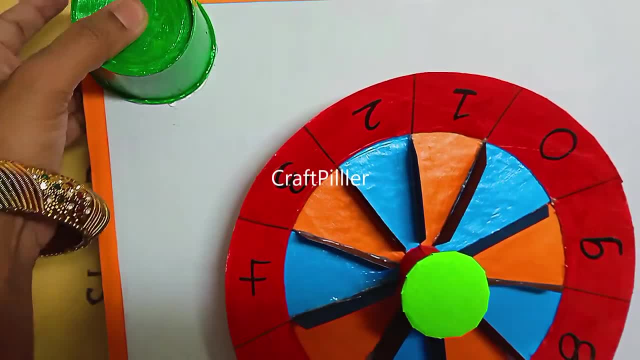 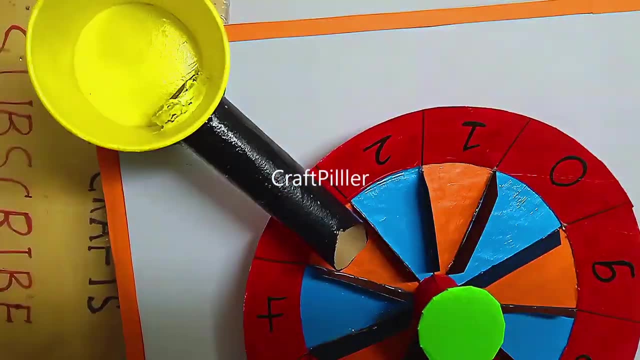 i'm playing sold out shows for a thousand faces. hey, give me that crown getting my way and to be put down. it ain't your place, all this my town. if i want that shit, then i'll get it. right now i'm losing it the noose it fits. i'm losing shit. a stupid myth. you choose to live or choose to. 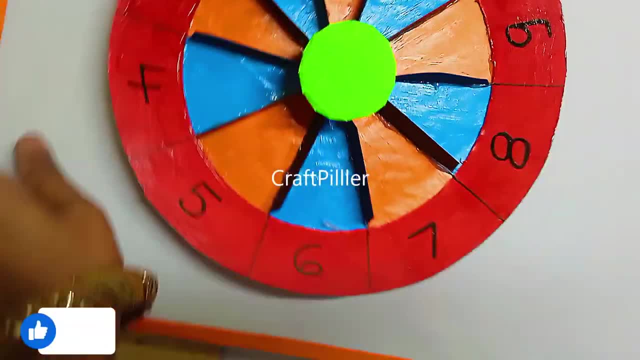 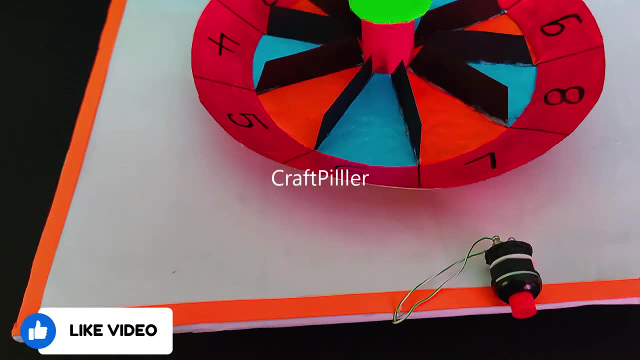 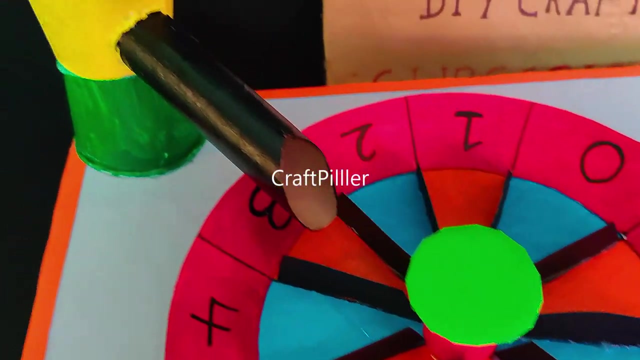 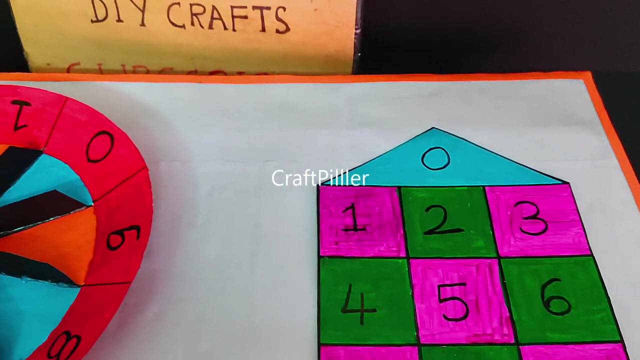 dip. you choose to fight or lose your grip and lose a gift. i feel like i'm losing my mind. is everybody in the world blind? please, lord, give me a sign, a sign. i feel like i'm losing my mind. is everybody in the world blind? please, lord, give me a sign. 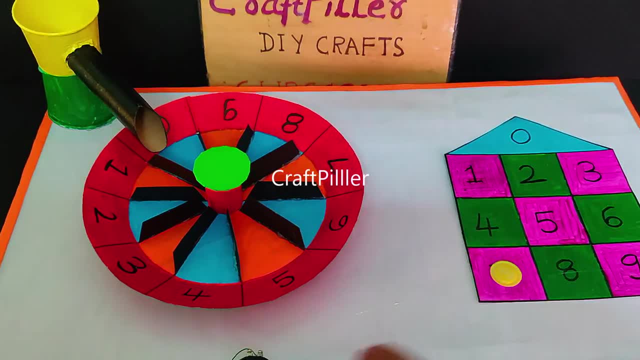 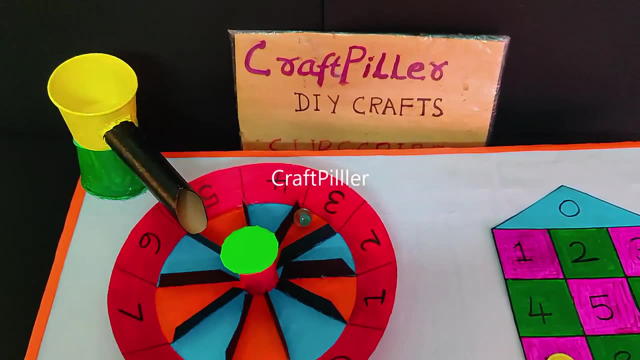 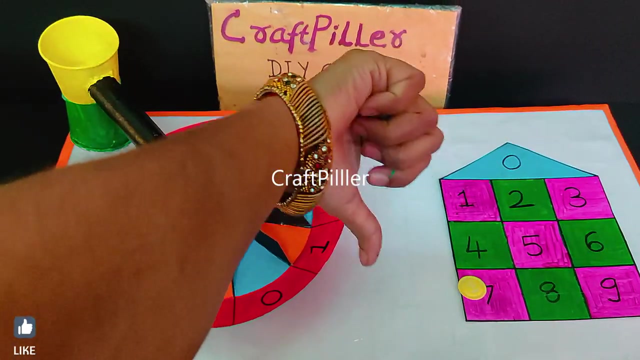 a sign. yo, there's no mercy in this world, just hunger, thirsty person, in different versions, each new. what they that shit worsens? why pull back the curtain and you'll see the different vermin. we all have different burdens that all seem to cause disturbance. yo do me a favor, don't treat me like a neighbor. don't need the different flavors of your problems. 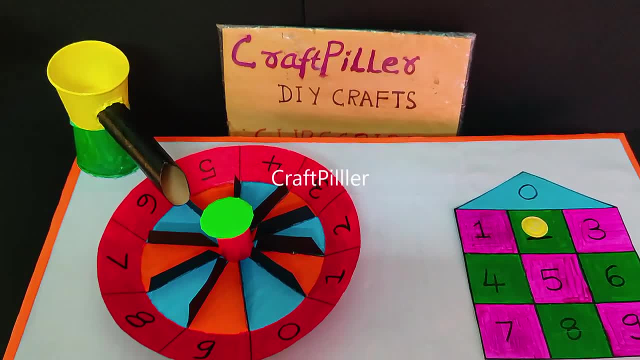 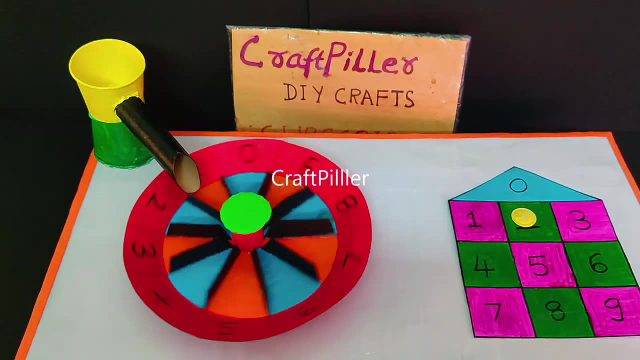 just to savor, i've got my own issues. i need a comb to get through. don't need to groan with you, just go get your own tissue. i feel like i'm losing my mind. is everybody in the world blind? please, lord, give me a sign. 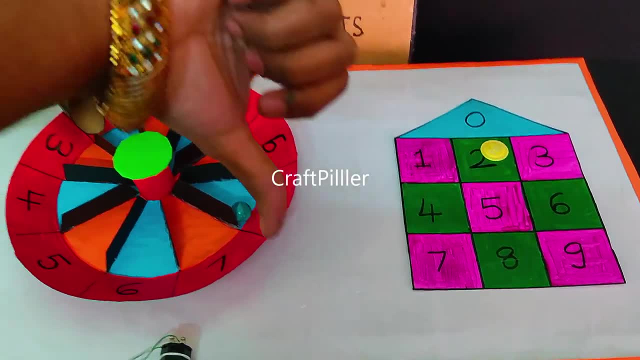 is everybody in the world blind? please, lord, give me a sign.